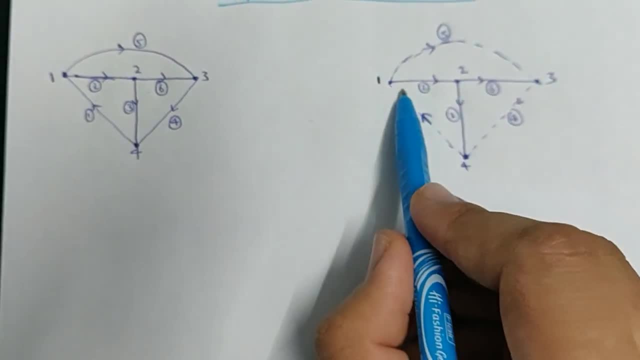 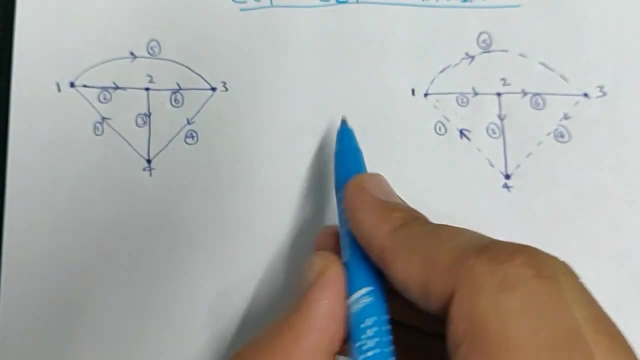 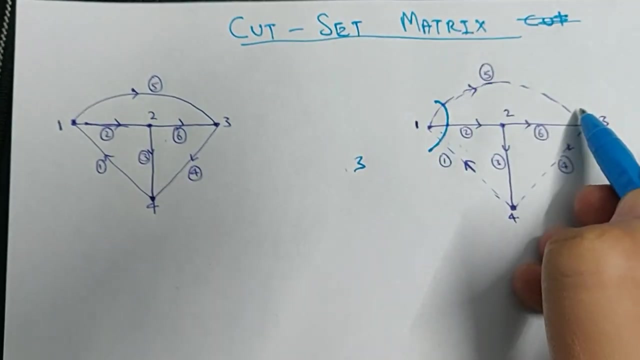 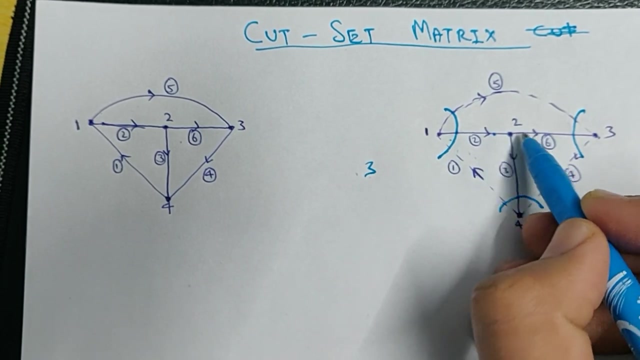 Okay, So we will have to cut these links. There are three links, So there will be three cuts present, Three cuts present. Okay, We will apply the cut at the node. Okay, So here is one cut. Here is another cut, Here is third cut. We can't apply a cut on this node because there are more than one branches, more than one link attached to this node. Okay, We can only cut the node where one link is attached. 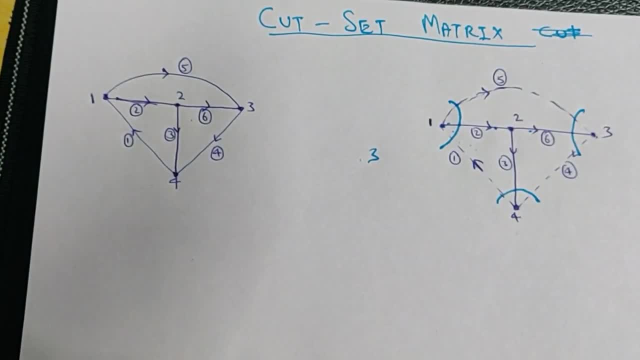 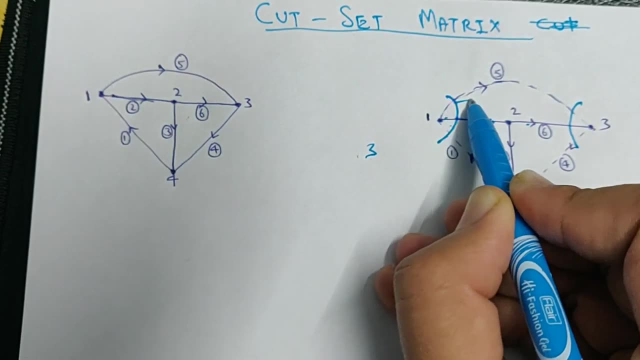 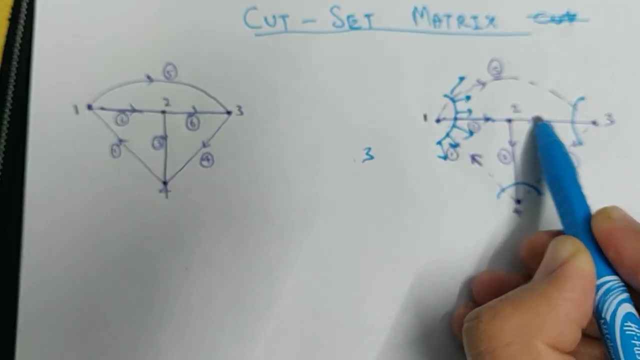 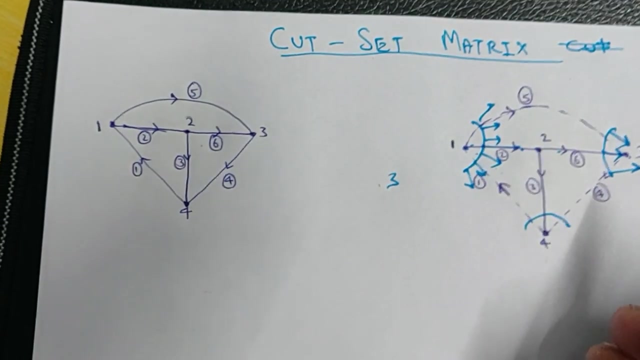 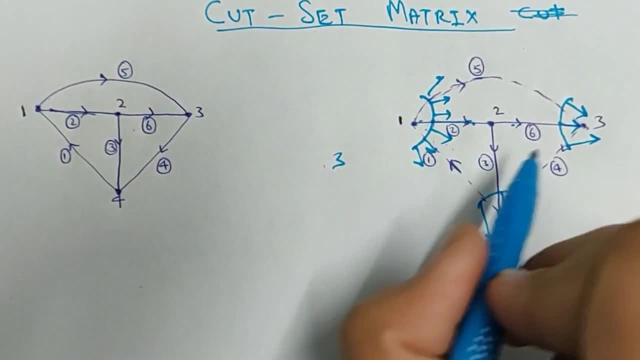 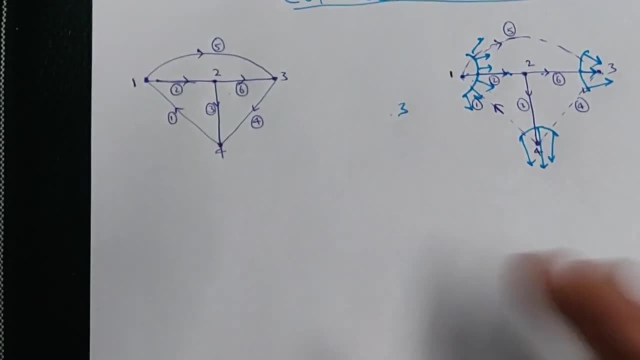 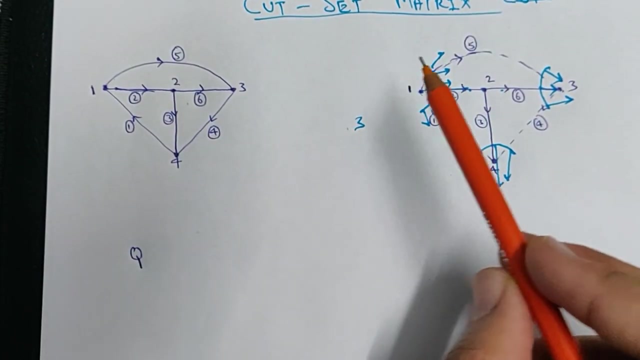 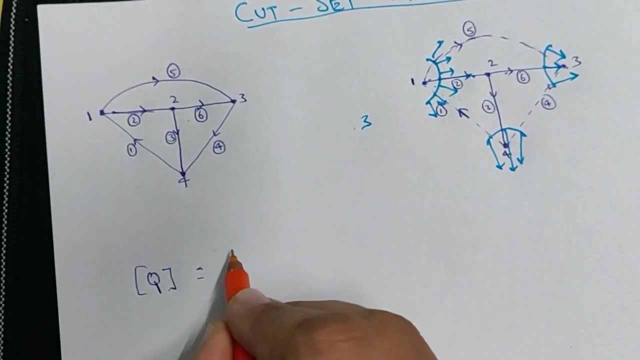 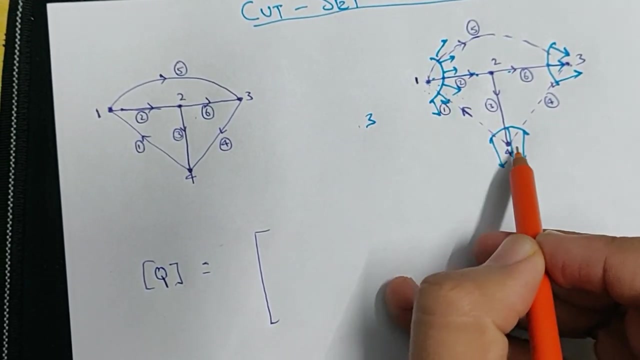 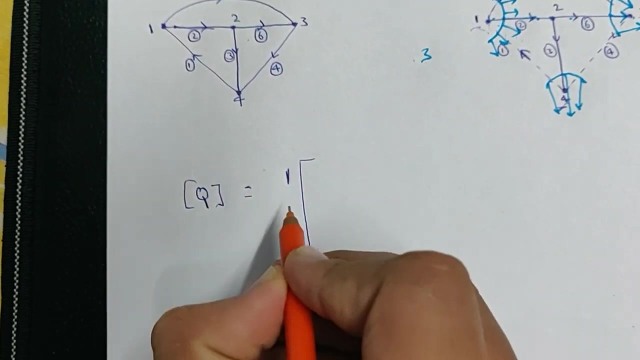 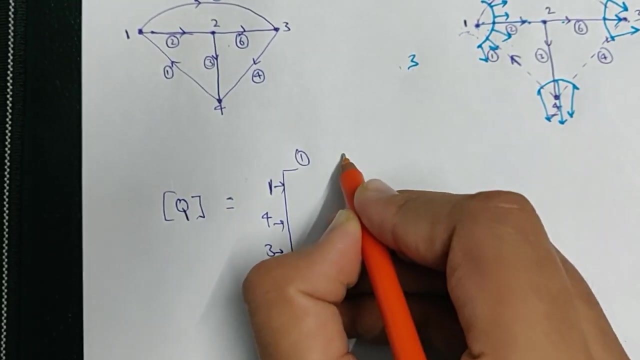 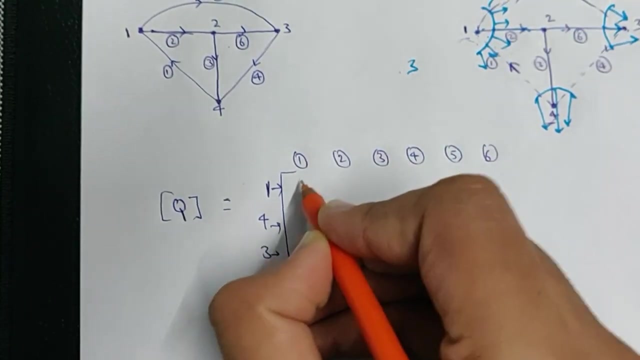 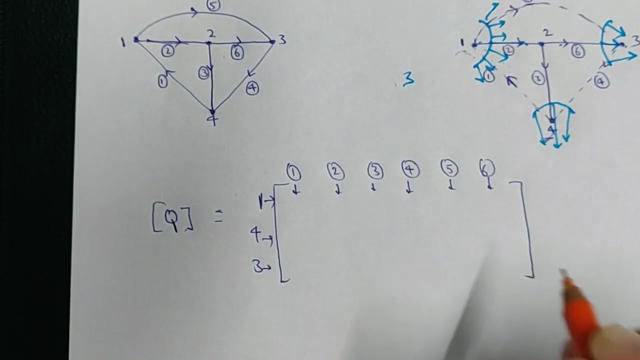 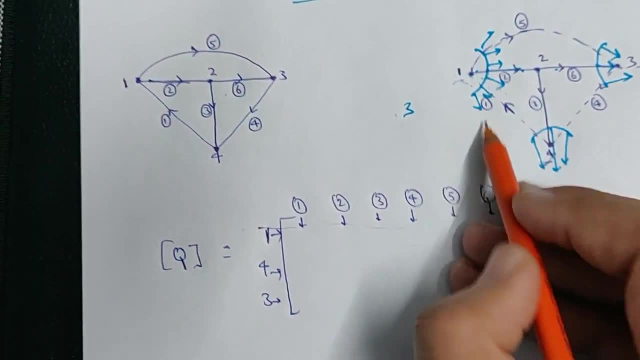 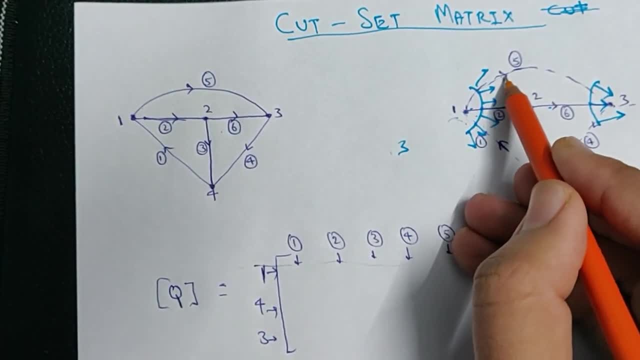 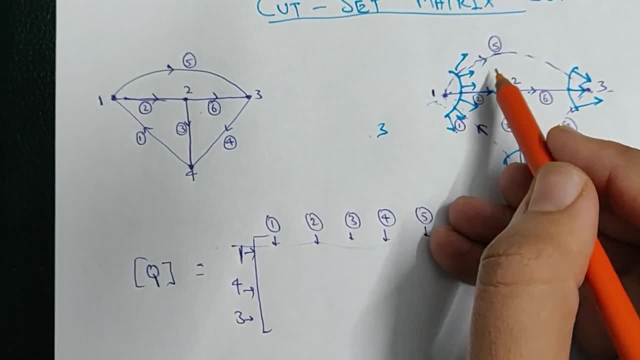 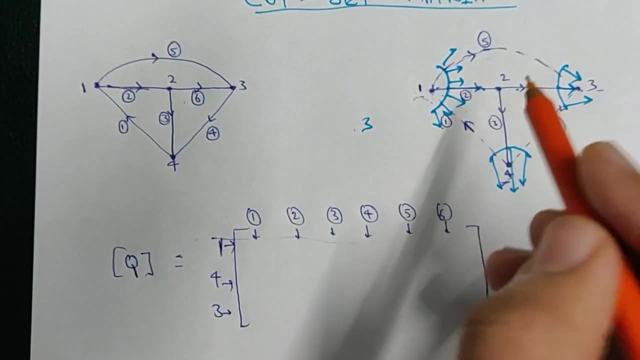 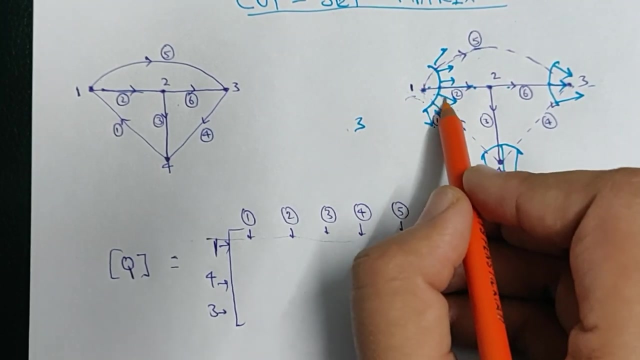 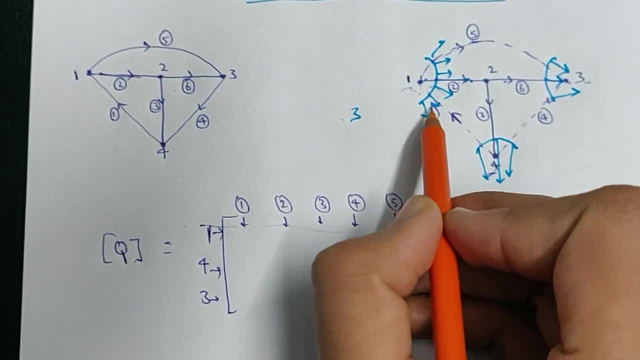 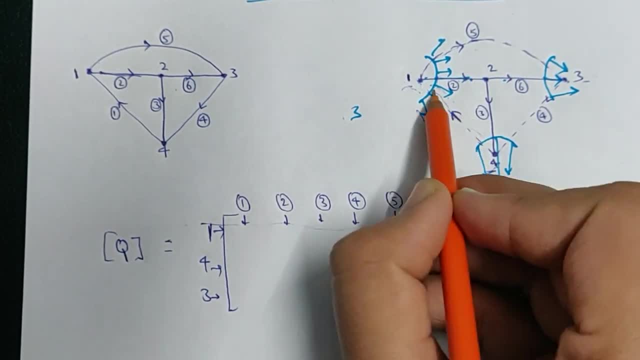 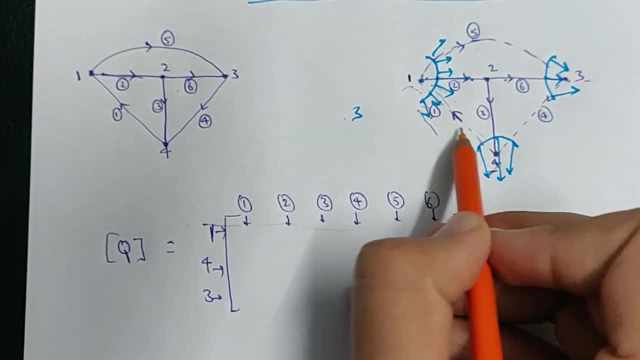 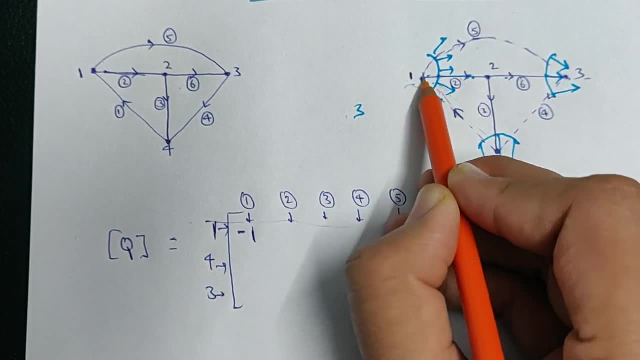 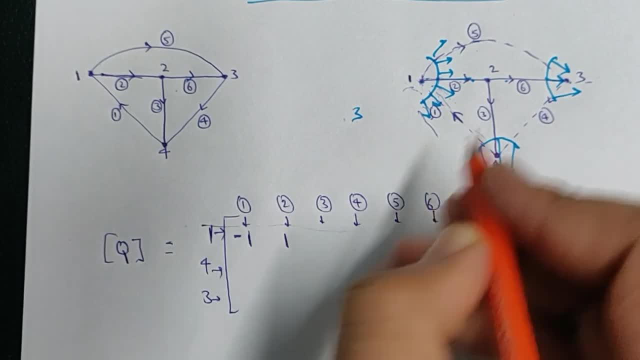 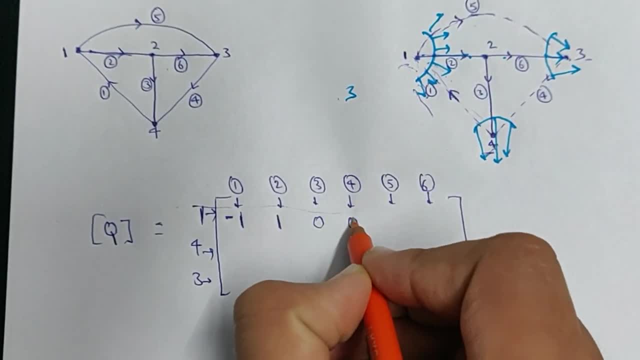 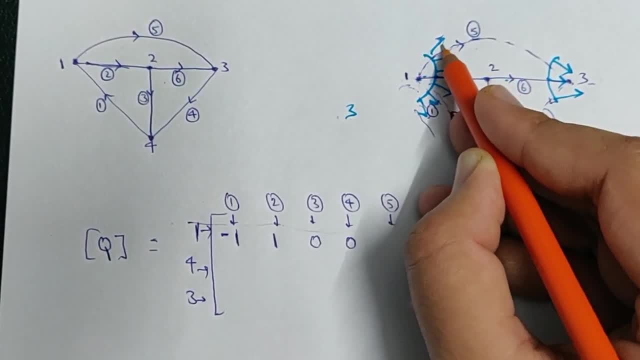 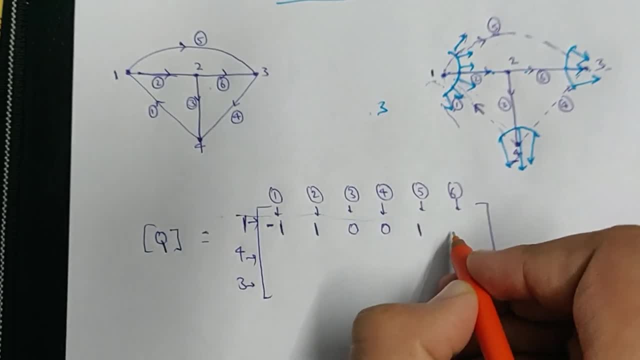 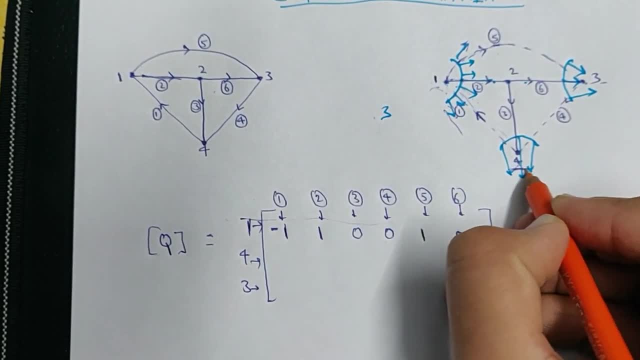 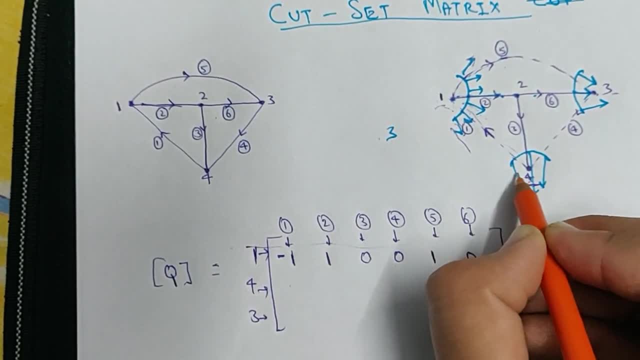 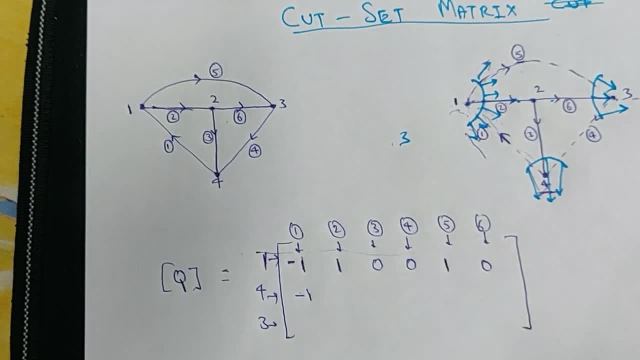 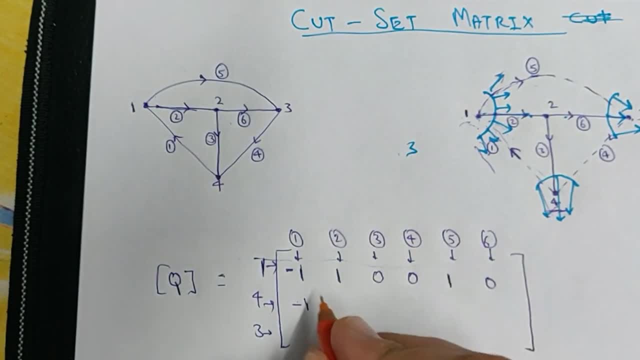 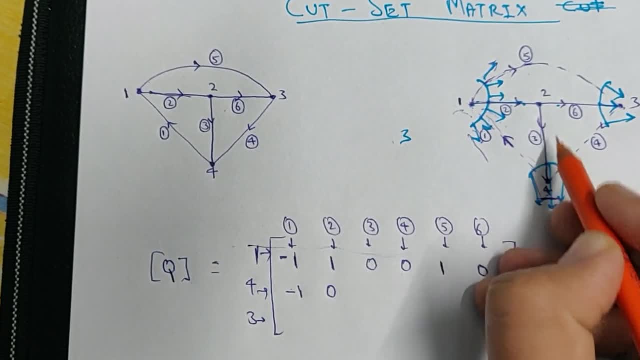 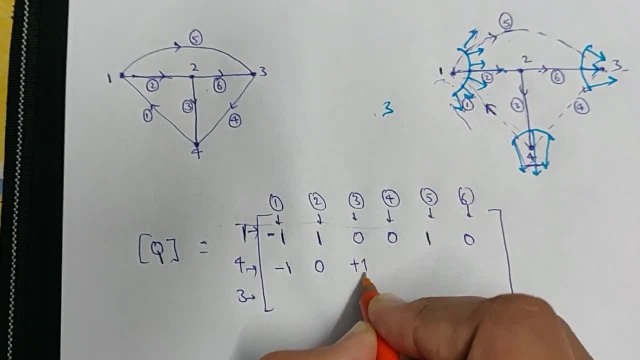 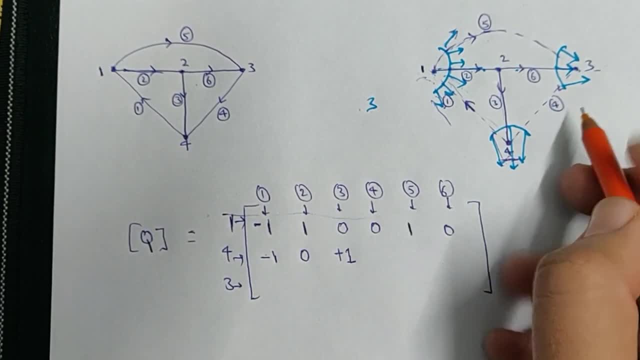 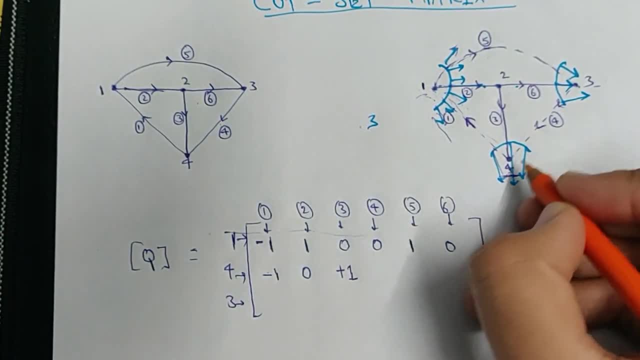 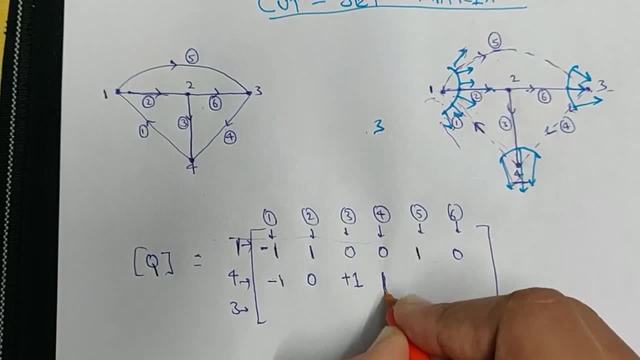 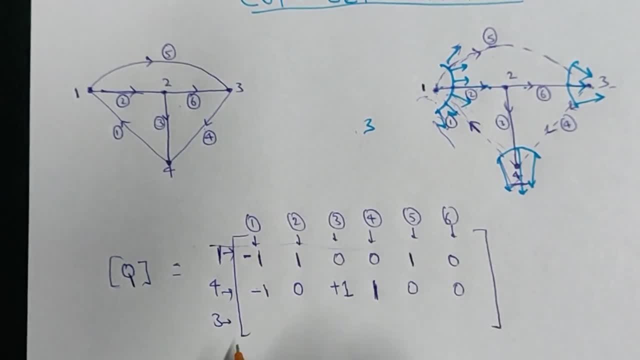 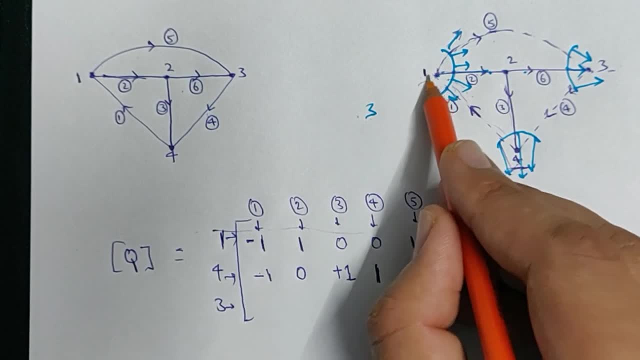 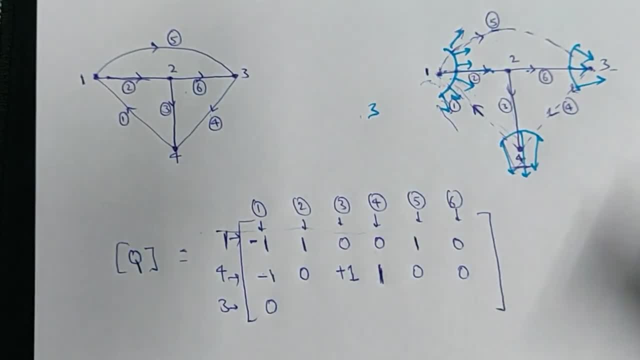 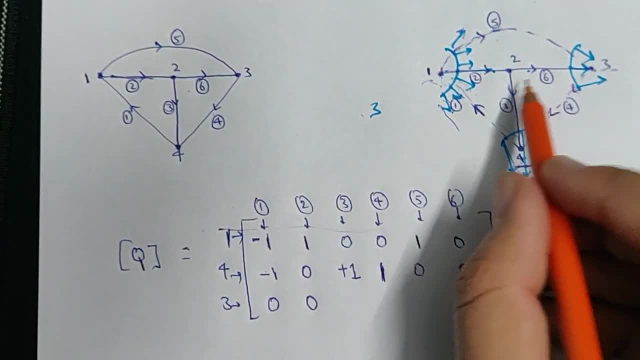 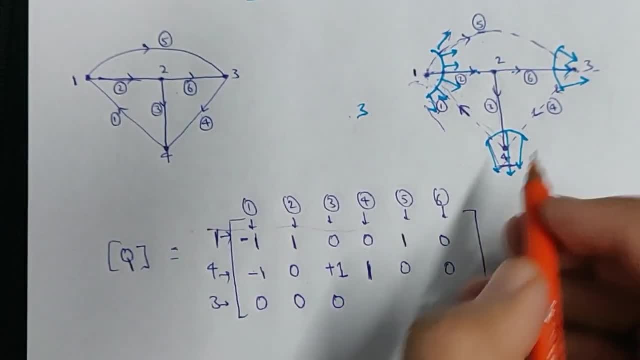 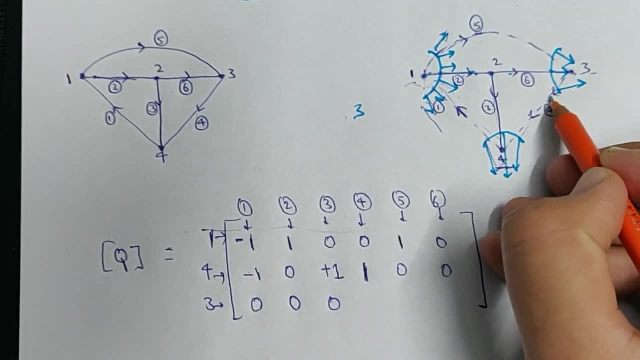 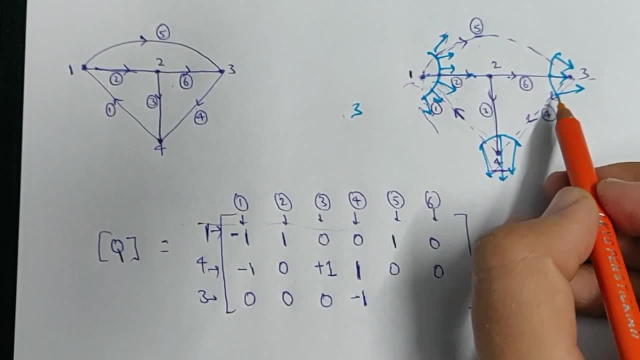 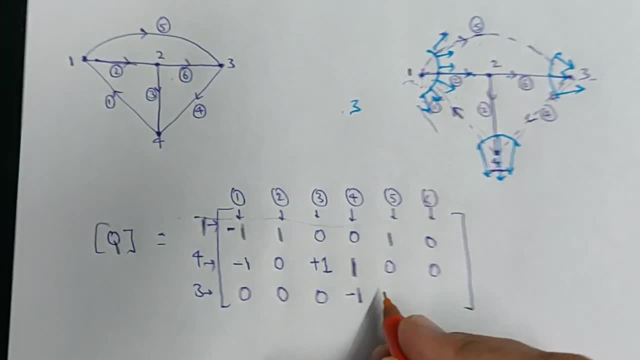 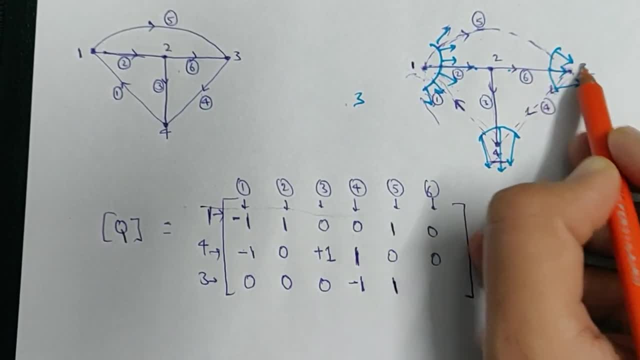 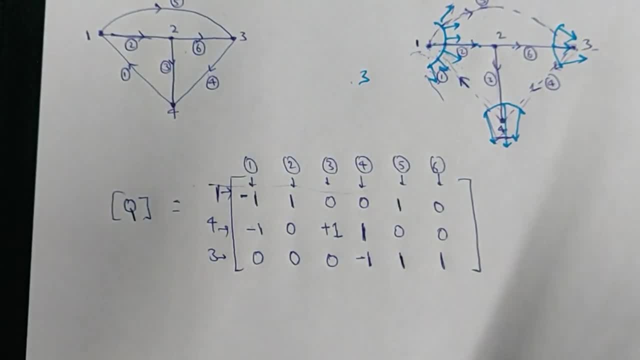 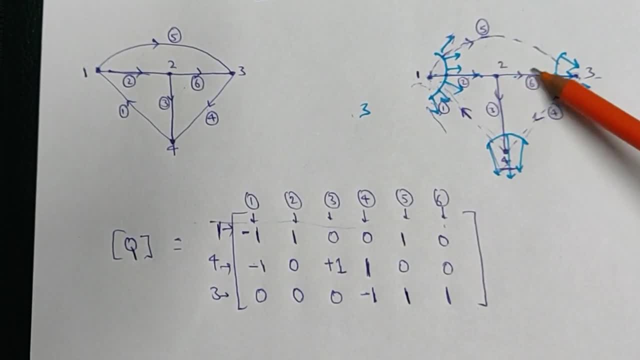 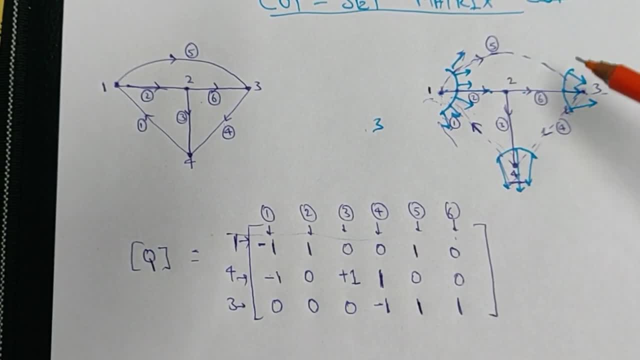 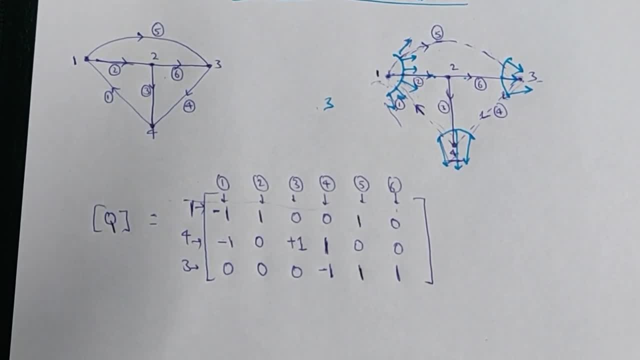